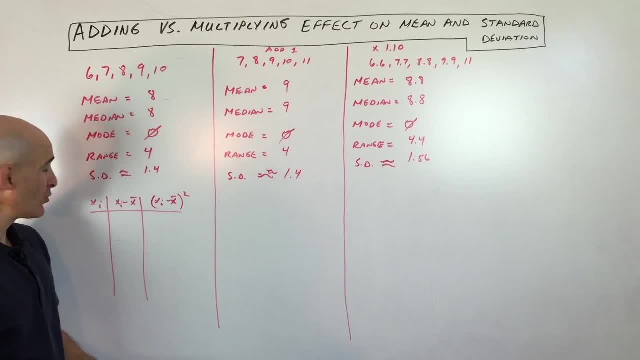 standard deviation. I would recommend setting up a table like this and I can show you how that works real quick. but basically what you would do is you would do 6,, 7,, 8,, 9, and 10.. You would take each. 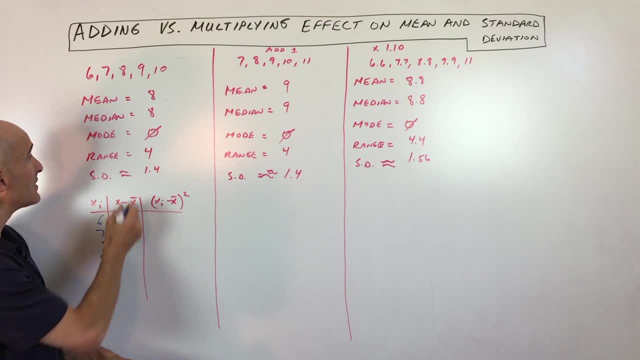 data point minus the mean. so 6 minus the mean, that's going to be 6 minus 8, which is negative 2, negative 1, 0,, 1, and 2.. Then you're going to square those deviations, that's 4, 1,, 0, 1, and 4.. You're going to add up those deviations squared. 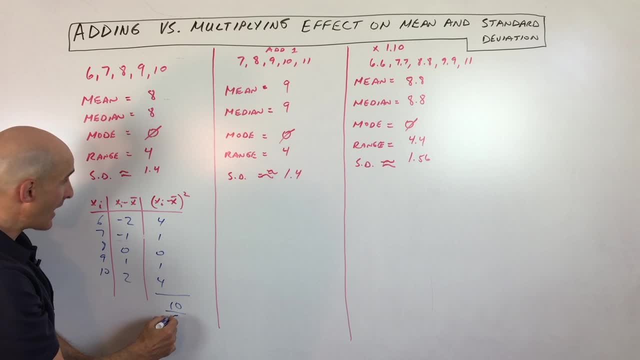 so that's going to be 10, divided by 5,, okay, and then you're going to that's the number of data points, and then you're going to take the square root. okay, so that's the square root of 2, which. 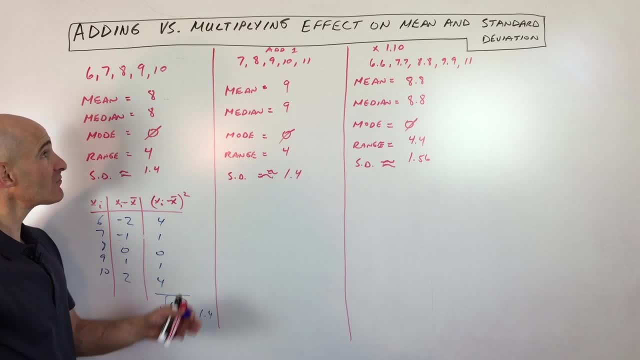 is about 1.4, so that's the standard deviation. Now let's just say that your teacher says: you know that was a really tough quiz. I'm going to give everybody an additional point. okay, so you're adding 1 to each of these. 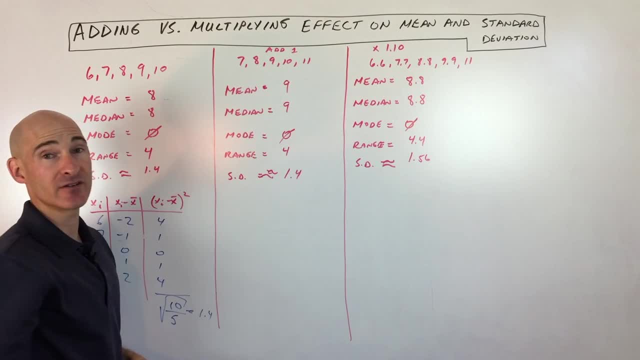 data points. Now the quiz scores look like 7,, 8,, 9,, 10, and 11,. okay, so now look what's happened to the mean. The mean has gone up by 1, see from 8 to 9.. The median has gone up by 1, 8 to 9.. 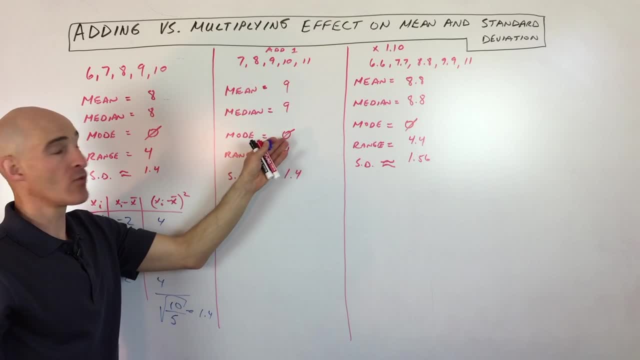 The mode still hasn't changed. okay, it would also go up by 1, but there was no mode in this example. but the range has not changed. See, if you do 11 minus 7,, that's 4,, just like 10 minus 6, that's 4,. 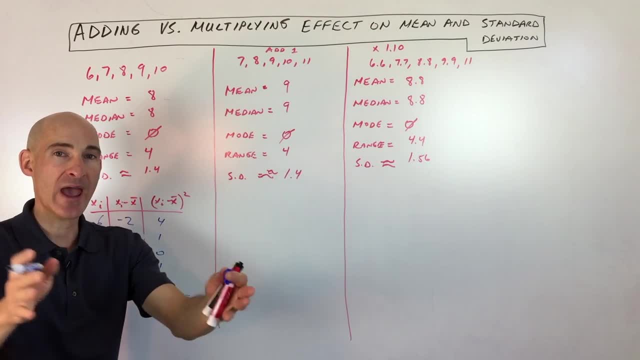 so the range gives you a sense of how spread out the data points are. When you add 1, everybody just shifts up one point. it doesn't affect the dispersion or the. you know how spread out the data points are. Same thing with the. 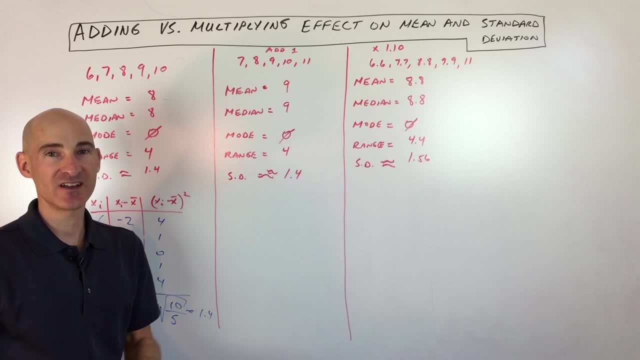 standard deviation, you can see it's exactly 1.4, I calculated that, you know, before I did this video. but again, the data, they're not spread out any further, everybody just shifted up one point. so again, the dispersion range and standard deviation give you a sense of how. 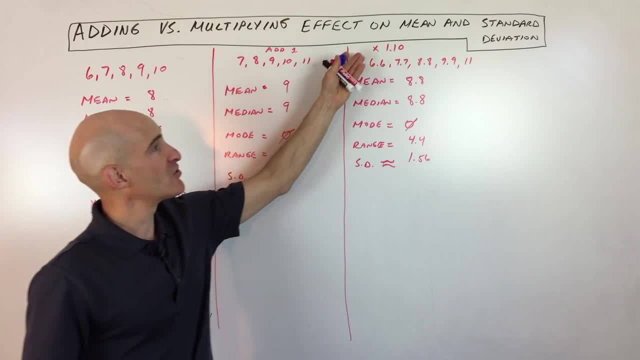 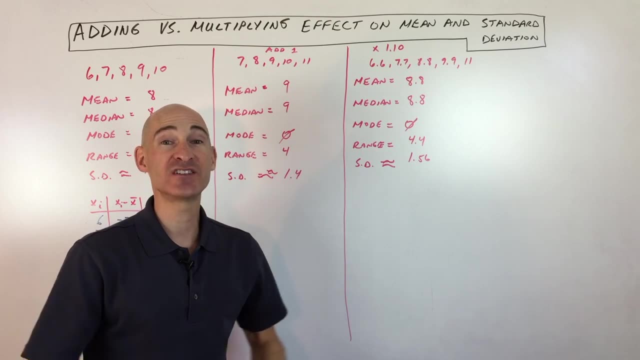 spread out. the data are, Those aren't changed. Now say, for example: your teacher again says: you know, that was a tough quiz. I'm going to scale the scores. I'm going to multiply everybody's score by 110%, so 1.10,. 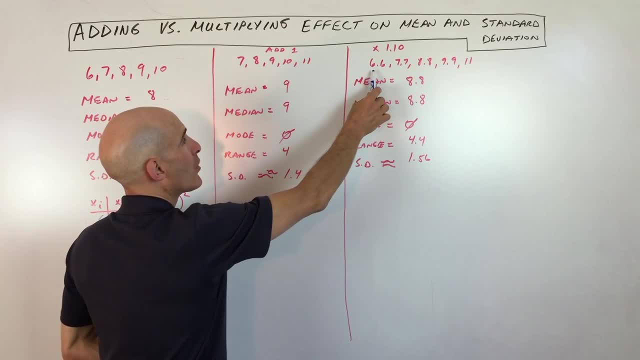 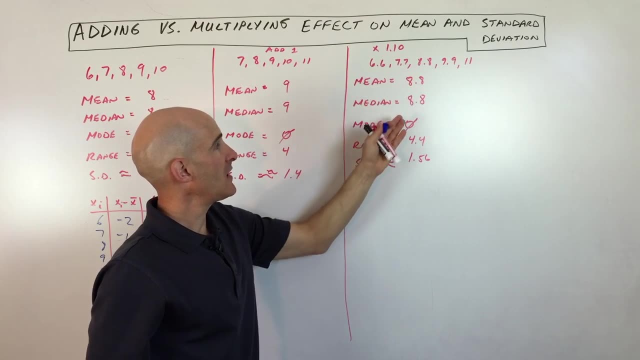 so I took all these data points here, I multiply them by 1.10, so you can see 6.6, 7.7, 8.8, and so on, and if you go to calculate the mean, you're going to get 8.8, the median, the middle one, is: